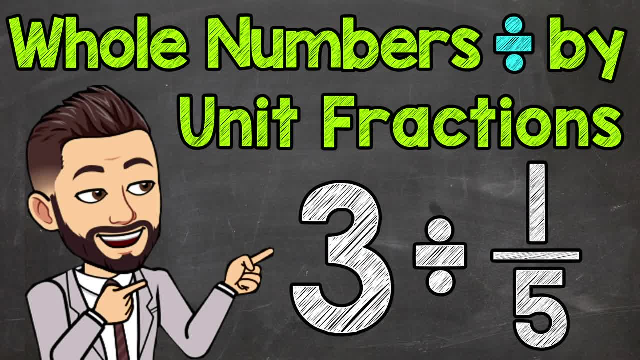 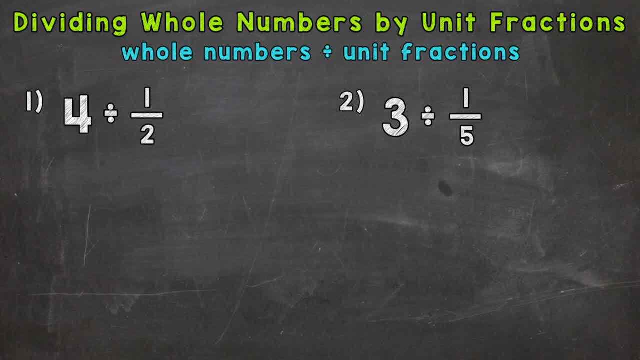 Welcome to Math with Mr J. In this video I'm going to cover how to divide whole numbers by unit fractions, and we have two examples here that we're going to go through together in order to get this down. And again, this is whole numbers divided by unit fractions. So let's take a look at number. 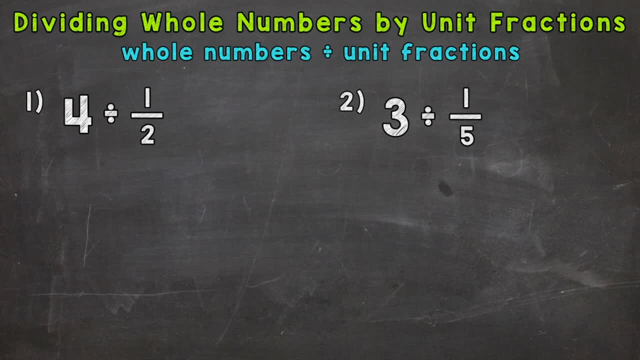 one where we have four divided by a half. Now there are three words that we need to keep in mind when we have fractions in division problems, and those words are: keep, switch and flip, And it is always in that order: Keep, switch, flip. So whether you have a whole number, 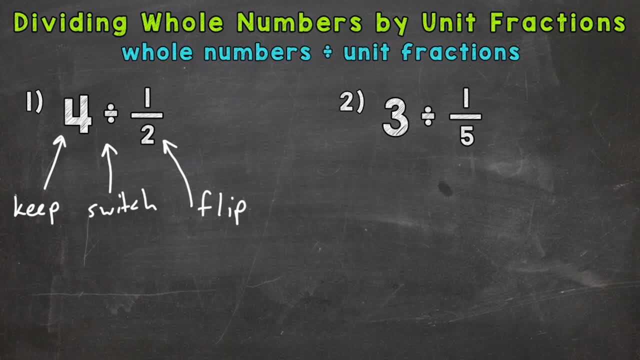 or fraction that comes first within your division problem. we keep it the same. So let's keep it as four. I'm going to put it in fractional form, so we have four divided by a half. So we're going to keep it in fractional form and we're going to 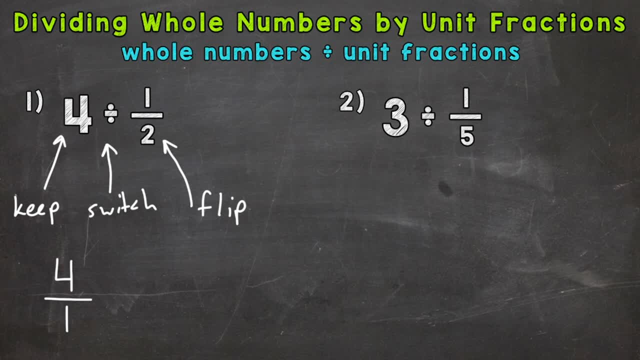 We have a numerator and denominator. You can do that by putting any whole number over 1.. Next, we switch this to a multiplication problem. So switch your division sign to a multiplication sign And since we're doing the opposite of division and changed it to multiplication, 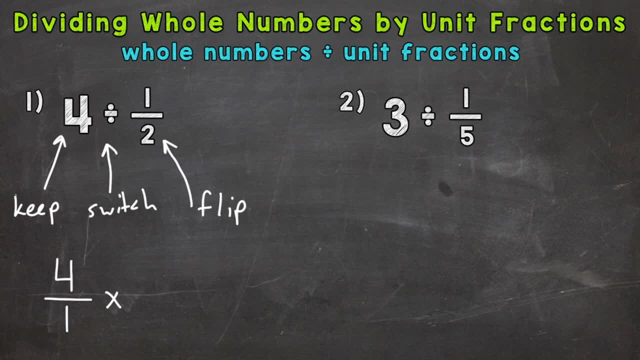 we need to flip that second number or fraction, whatever the case may be- in that problem in order to keep this problem equivalent to the original division problem. So the 2 is going to become the numerator and the 1 is going to become the denominator. 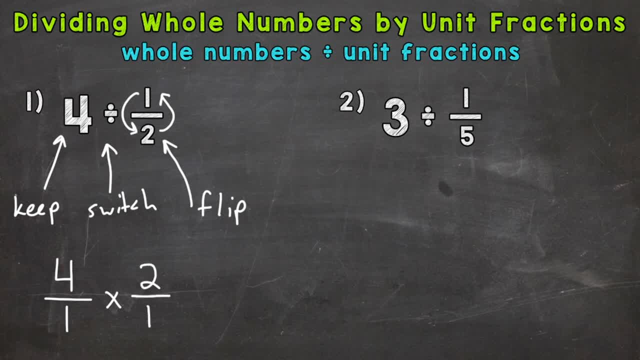 So we have 2 over 1.. Now we can multiply straight across: 4 times 2 is 8 and 1 times 1 is 1.. We have an improper fraction, so we divide. How many groups of 1 can we pull out of 8?? 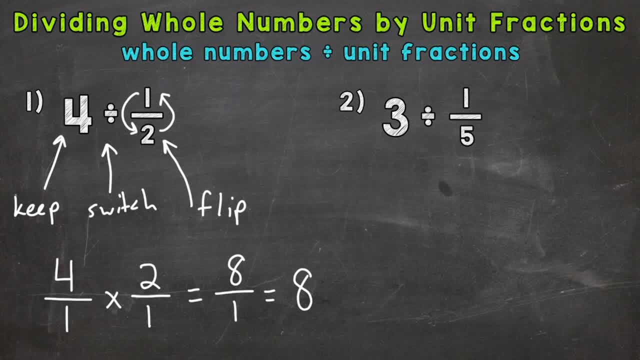 Well, 8.. Or you can think of it as well: we have a whole number over 1, so it's just going to be that whole number And our answer is 8.. So let's take a look at our original problem. 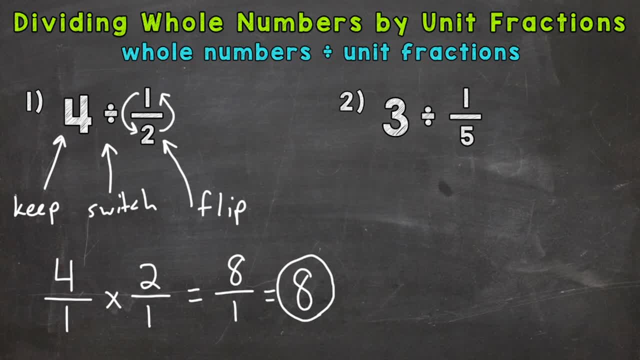 So we started with a 4,, a whole 4, and we have a division problem and we got an answer greater than what we started with. That's because if you divide by a fraction less than a whole, you get something greater than what you started with. 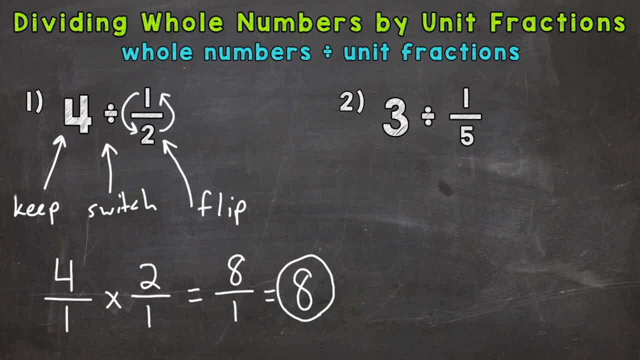 I'm going to draw a picture here real quick to show us how we got 8.. So let's see, Let's start with 4 holes here And I'm just going to use circles. You can really use any shape, but circles are pretty easy to work with. 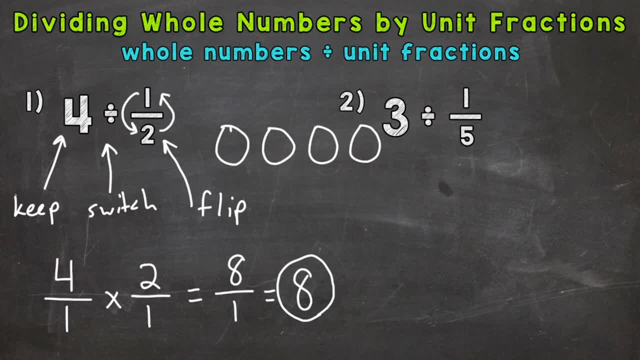 Now we're going to divide each of those holes in half. All right, Let's see how many pieces we have once we divided each hole in half. Well, 1,, 2, 3,, 4,, 5,, 6,, 7, and 8.. 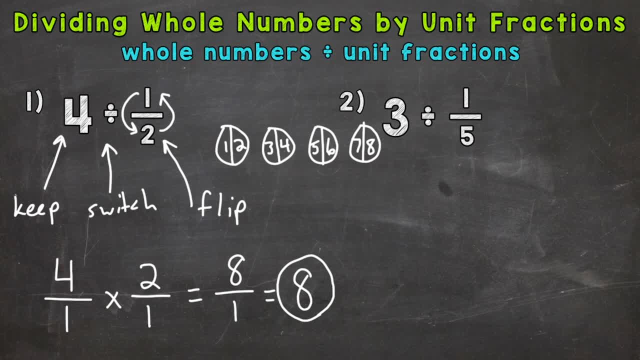 So we start with 4 holes, divide it in half and we ended up with 8 pieces And that model matches our answer. Now I have a whole video on modeling these types of problems. I have that link down in the description if you want to learn more about modeling these problems. 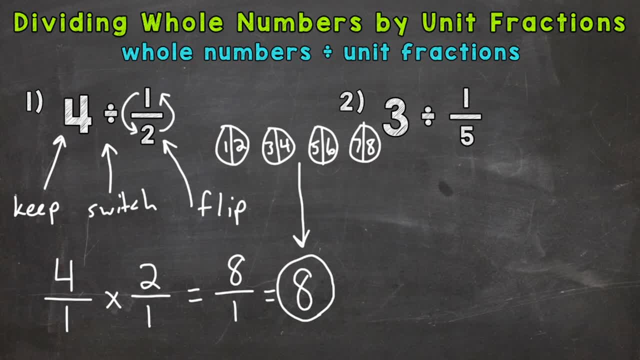 and get a deeper understanding. So let's go to number 2, where we have 3 divided by 1. fifth, So again the three most important words: when we have fractions within a division problem, keep switch, flip. So let's keep the 3.. 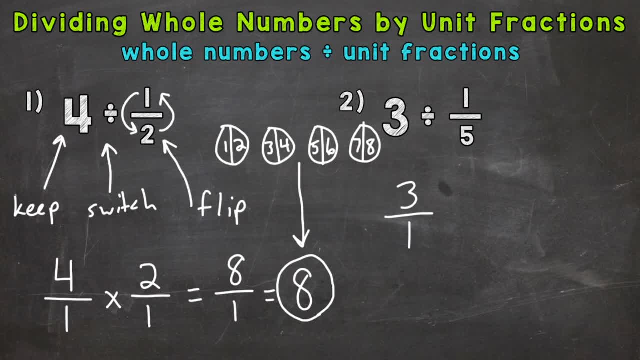 Keep the 3 as is. We can put it over 1 to put it into fractional form, but that still has the value of 3.. So we are keeping it as 3.. Switch to multiplication and flip your second fraction or number to keep this problem equivalent. 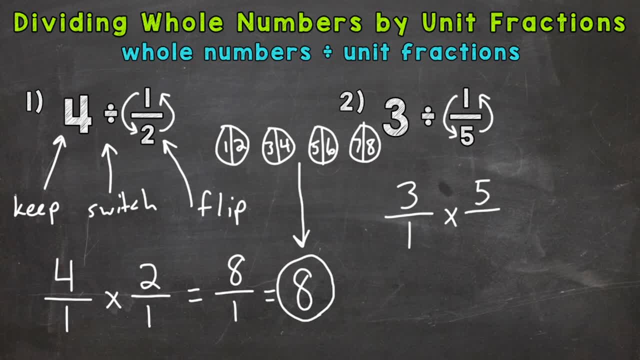 to our original problem. So the 5 is on top and the 1 is below, And now we are good to go. We can multiply straight across, So we get 15 over 1, which is 15 holes. So we started with 3 holes. divided each of those 3 holes into 5 pieces or fifths. 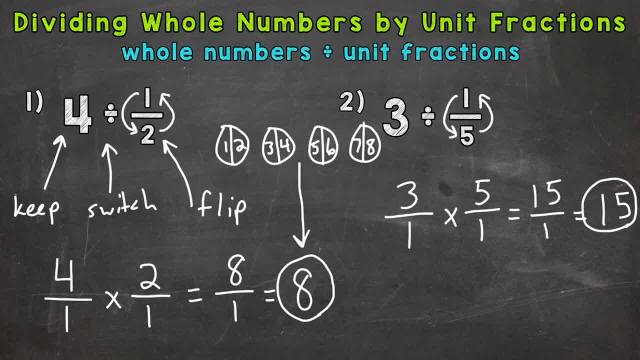 and we end up with 15 pieces. So there you have it. There's how you divide whole numbers by unit fractions, Like I mentioned in number 1, with that modeling video I have. I have a handful of other dividing fractions videos with models and without models. 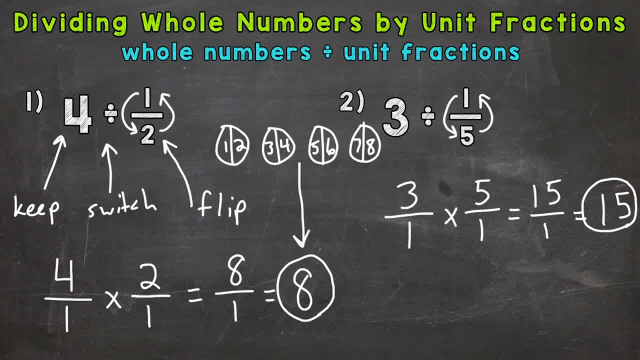 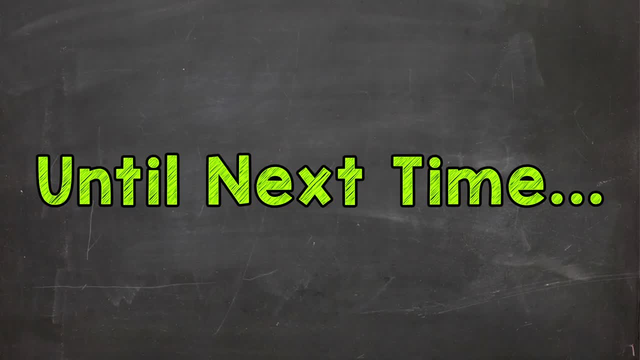